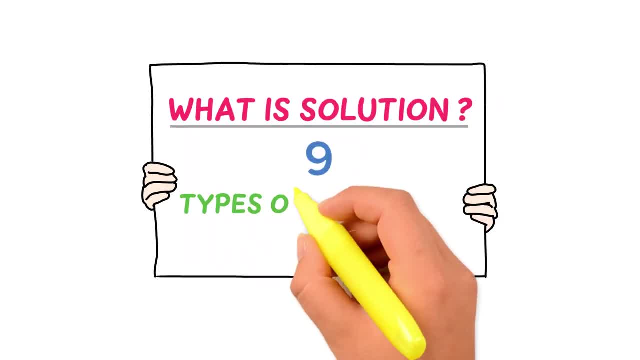 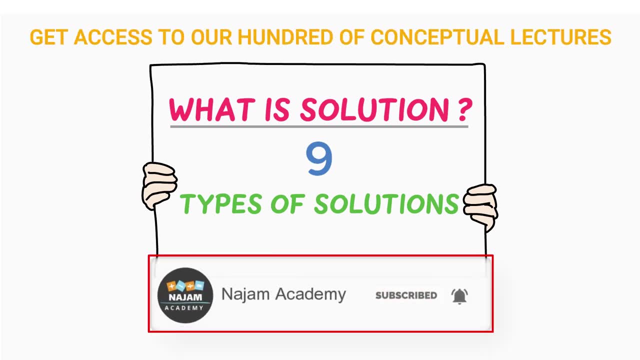 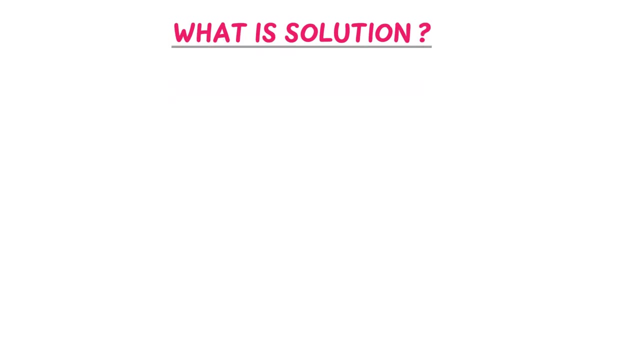 What is solution? What are the nine types of solution? Before starting the lecture, click on the subscribe button and get access to our hundred of conceptual lectures for free. Now, what is solution? Well, a homogeneous mixture of two, or more than two, substances. 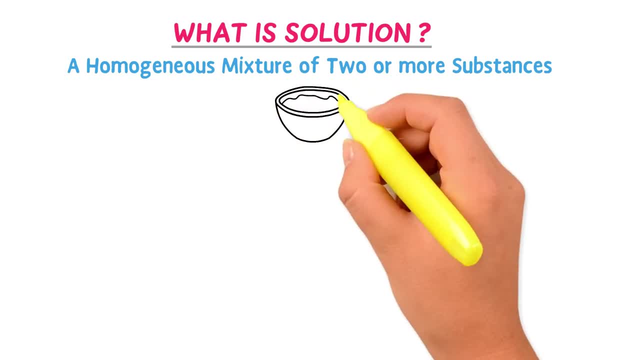 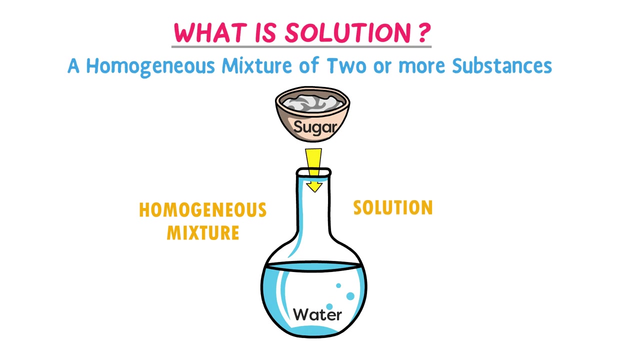 is called solution. For example, when you add sugar to the water, you form a homogeneous mixture of sugar and water. This homogeneous mixture is called solution. Usually, a solution is made up of two components: solute and solvent. Solvent is the component of solution which is 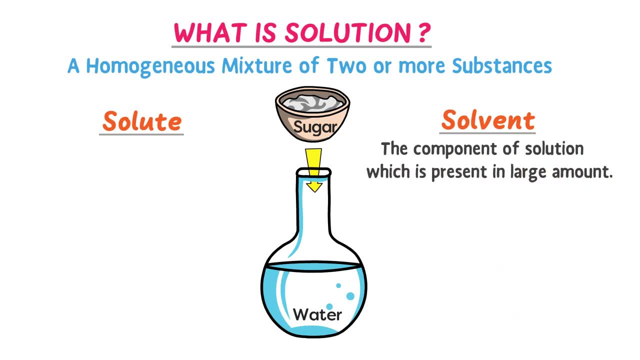 present in large amount and the solution is the component of solution. So what is solution, While solute is the component of solution, which is present in small amount, and the solution? For example, in this solution, water is solvent and sugar is solute. Remember that we are going. 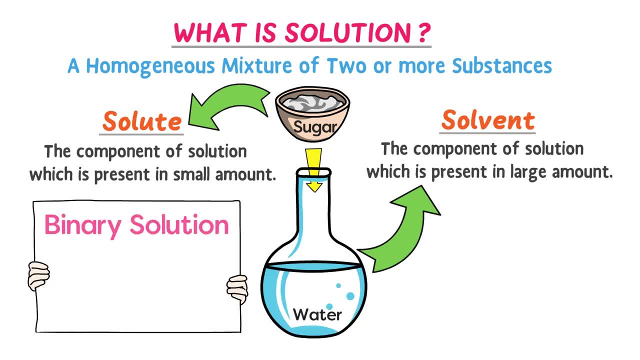 to learn about binary solutions in this lecture. A solution which is made up of two components is called binary solution. For example, this solution is made up of two components: is made out of sugar and water, So it is also called binary solution. 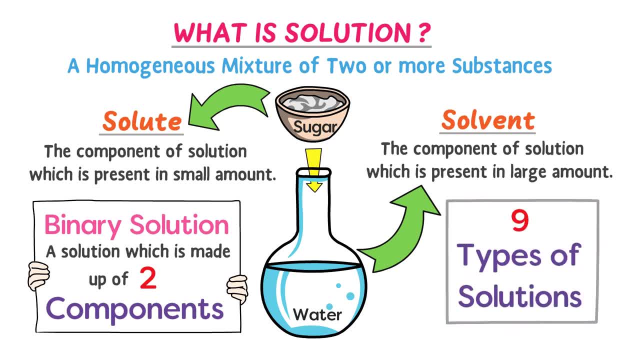 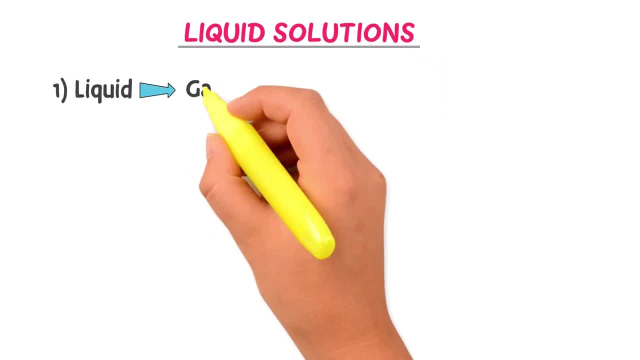 Now, what are the nine types of solutions? Firstly, we will learn the three different types of liquid solutions, like dissolving liquid in gas, liquid in liquid and liquid in solid. Remember that in all these three solutions, liquid is taken as a solute and then dissolved. 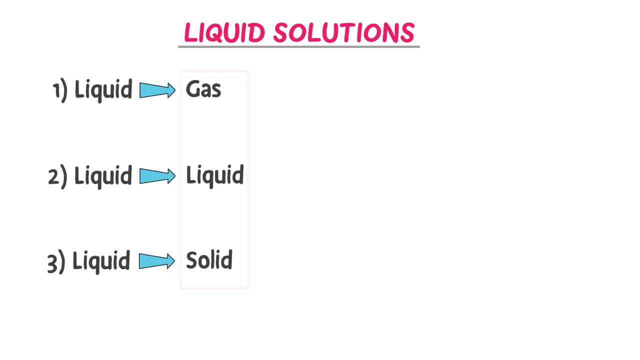 in these different solvents. The example of dissolving liquid in gas solution is cloud or fog. We know that cloud or water vapors and air. Secondly, the example of liquid in liquid solution is dissolving alcohol and water. Thirdly, the example of liquid in solid. 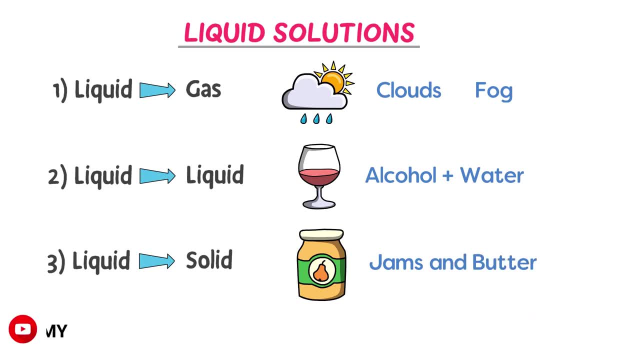 solution is jams, butter or cheese. 3. y a, min a, y, b, e. Remember that clout and fog are the solutions in which liquid is dissolved and gas. Alcohol plus water is the solution in which liquid is dissolved and liquid, while jams. 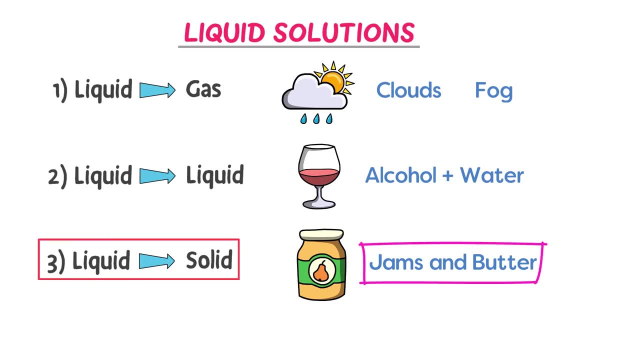 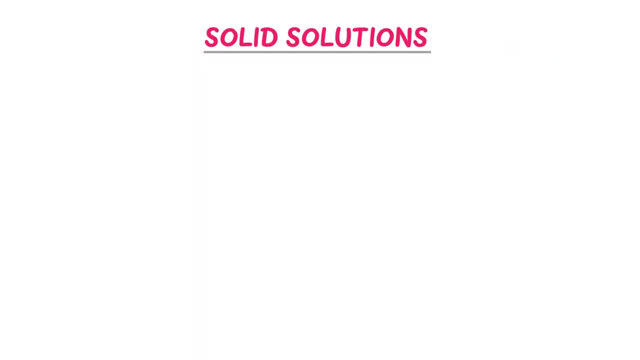 and butter are the solutions in which liquid is dissolved and solid. Now let me teach you the three different types of solid solutions, like dissolving solid in gas, solid in liquid and solid in solid. Remember that in all these three solutions, solid is taken as a solute and then dissolved. 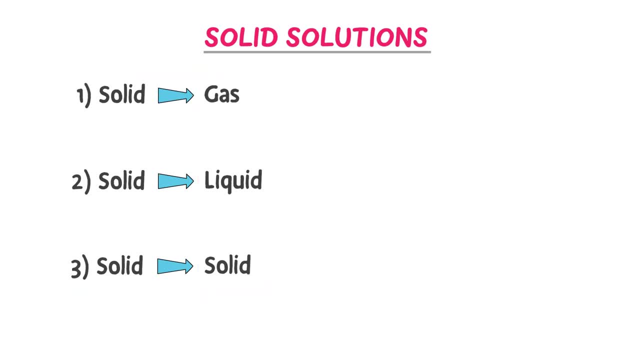 in these three different solvents. The example of solid in gas solution is smoke. We know that smoke contains carbon particles and air. Secondly, the example of solid in liquid solution is smoke. It contains sugar and water. Thirdly, the example of solid in solid solution is alloy. 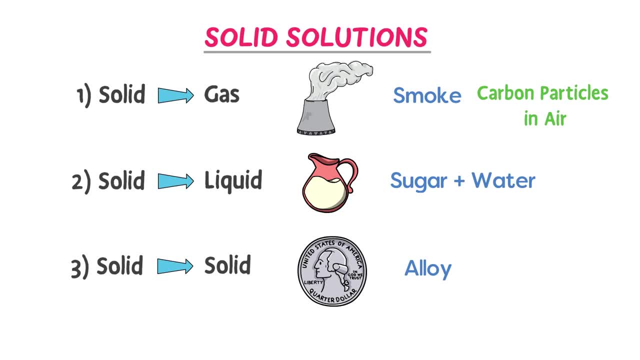 We know that alloy is made up of two or more metals, like alloy of copper and tin. Thus, remember that smoke is the solution in which solid is dissolved in the gas. Sugar and water is the solution in which solid is dissolved in the liquid, while alloy is. 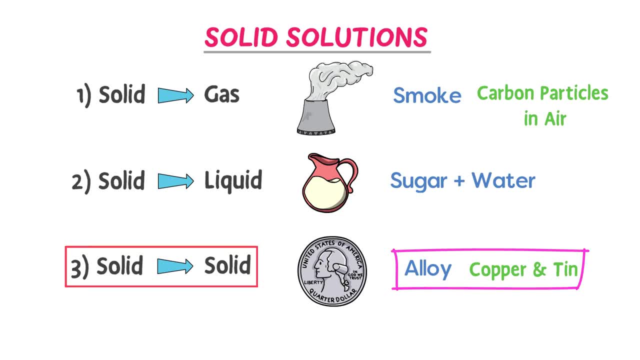 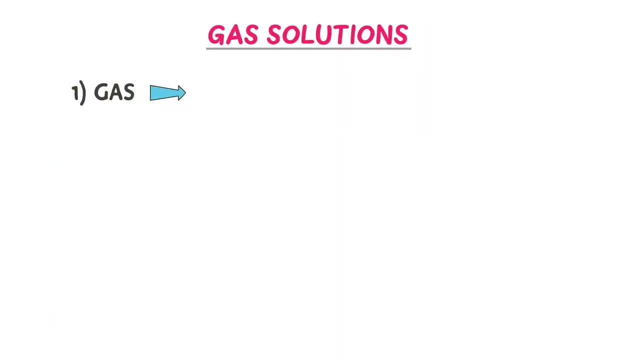 the solution in which solid is dissolved in the gas. Finally, let me teach you three different solutions of gases, like gas in gas, gas in liquid and gas in solid. Remember that in all these three solutions, gas is taken as a solute and then dissolved. 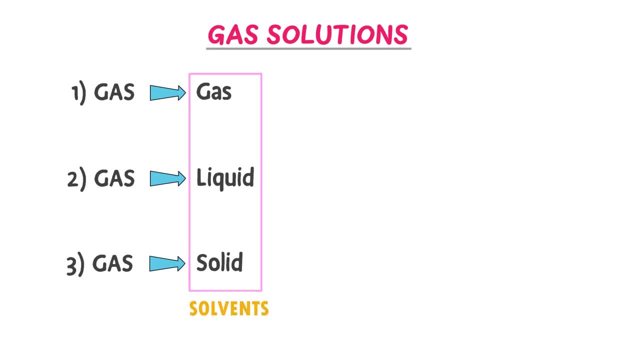 in these three different solvents. The example of gas in gas solution is air. We know that air is a hot solution. The example of gas in gas solution is air. Air is a homogeneous mixture of different gases like nitrogen gas, oxygen gas, noble. 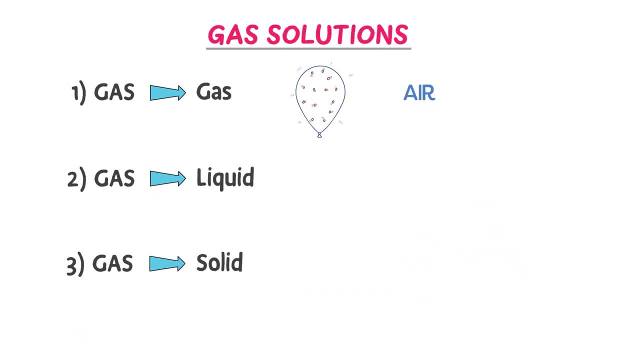 gases, etc. Secondly, the example of gas in liquid solution is carbonated drinks. In the carbonated drinks, carbon dioxide is dissolved in water. Thirdly, the example of gas in solid is hydrogen gas absorbed by the platinum sheet or marshmallow.